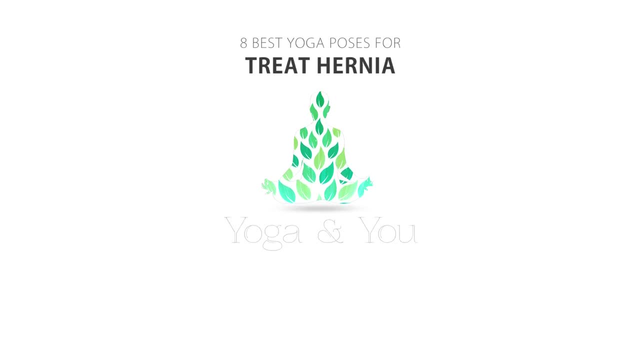 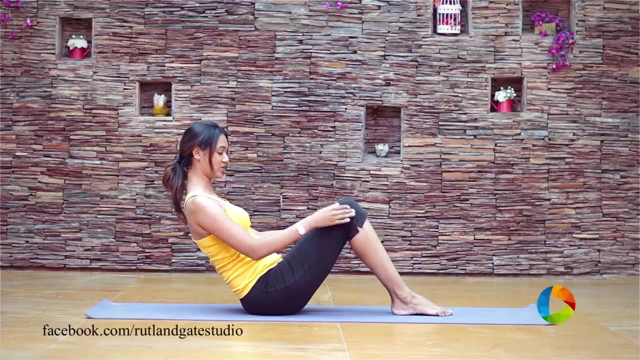 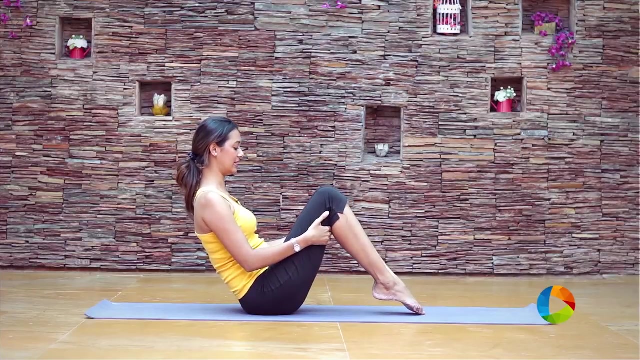 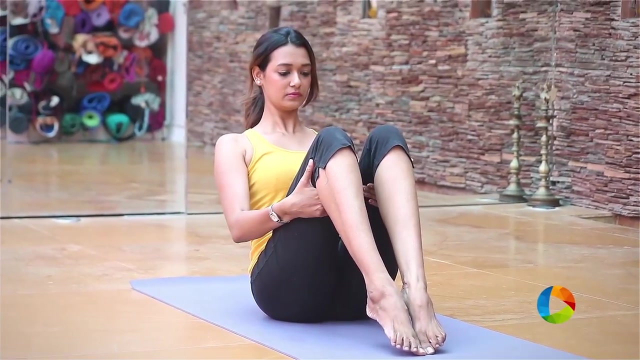 Roll your shoulders back and slowly lean all the way back, just like this, So keeping your back strong and nice and sturdy, And from here, as you inhale, lift your legs slowly off the mat and keeping your upper body position straight, right there and slowly keep breathing. 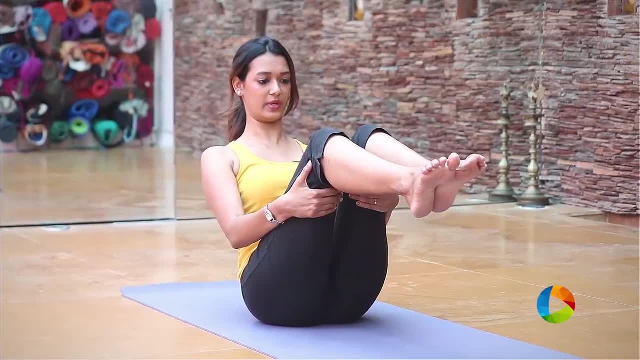 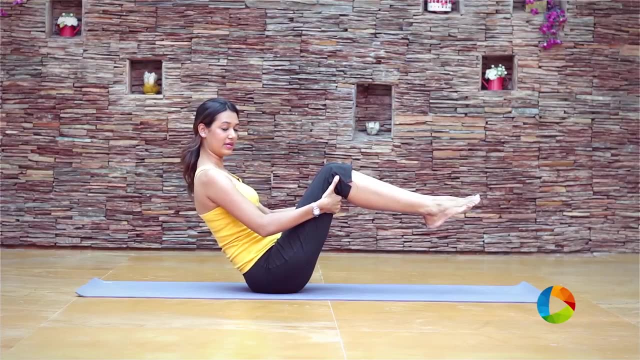 normal breath here, Inhale, lift your legs all the way up. If you want to hold your legs like this, you could always support your arms just like this behind your thighs. and if you want to leave the arms and still hold the posture, then slowly release your arms to the. 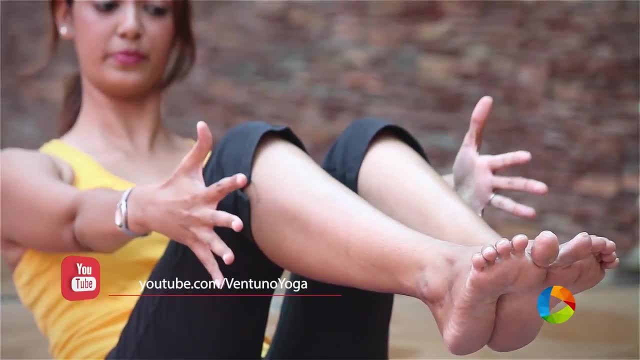 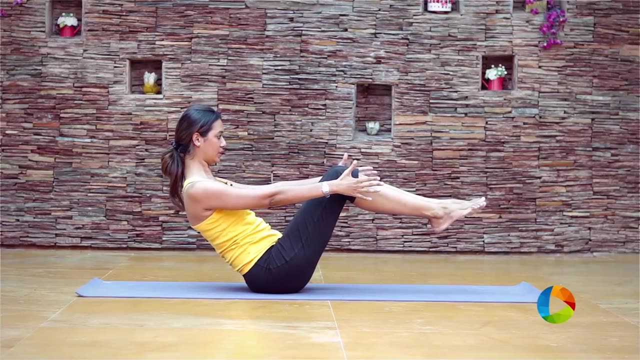 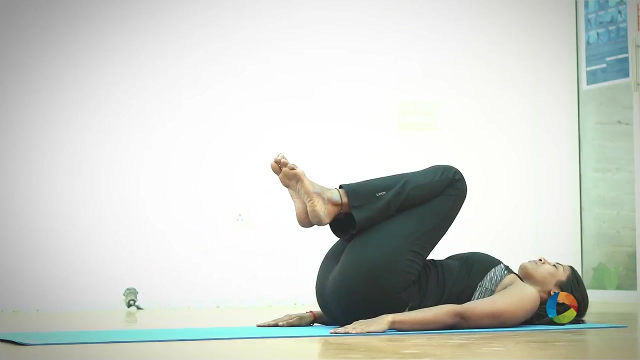 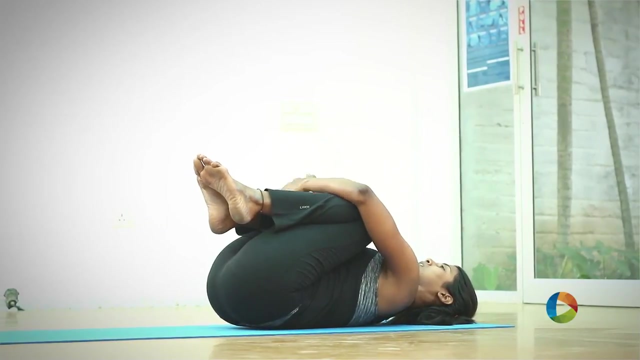 sides of your body and hold the posture, not your breath. Remember to breathe for 5,, 4,, 3,, 2, 1.. Now gently take both the knees towards the chest. Interlock your hands. If you want more squeezing of your abdomen, you can hold both the sides of your elbow. Pull the navel inside. 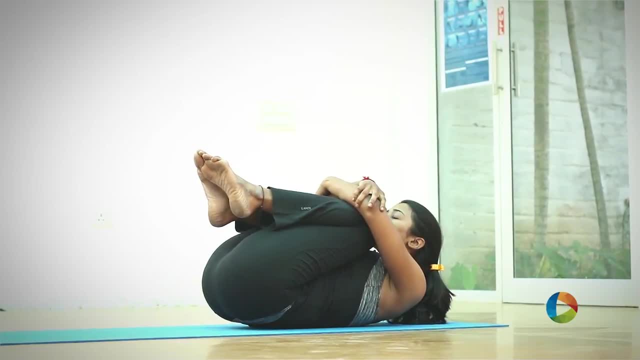 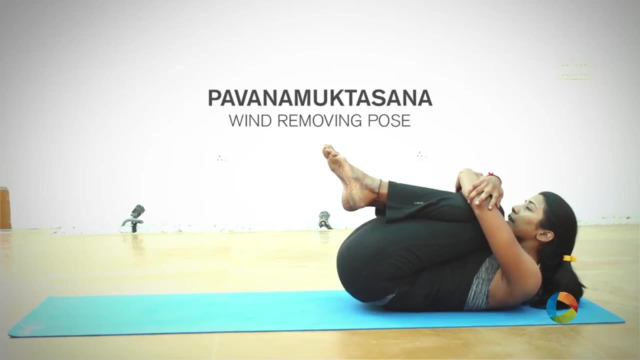 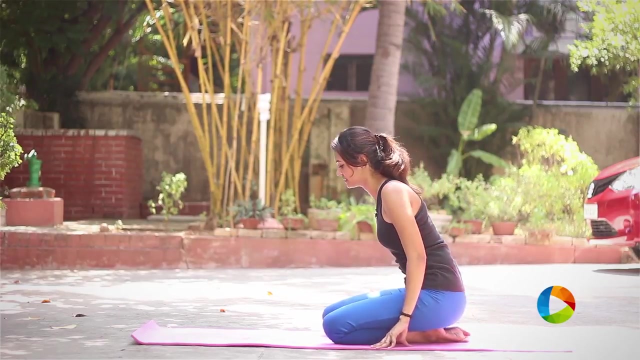 as you exhale, Try taking the chin towards the knee. Don't take your forehead to the knee, then it will be hurting your neck. So begin by sitting in Vajrasana and what you want to do is basically stand onto your knees and widen your legs. really nice. Bring your palms facing down, your fingers facing. 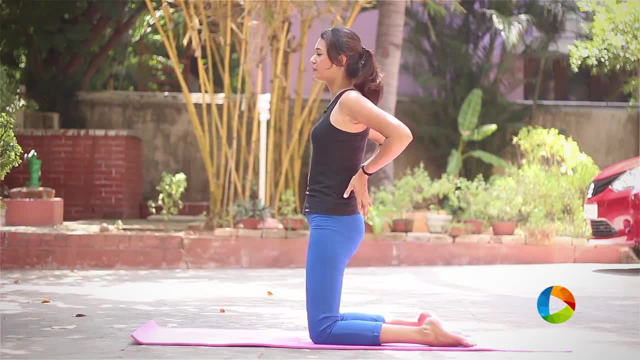 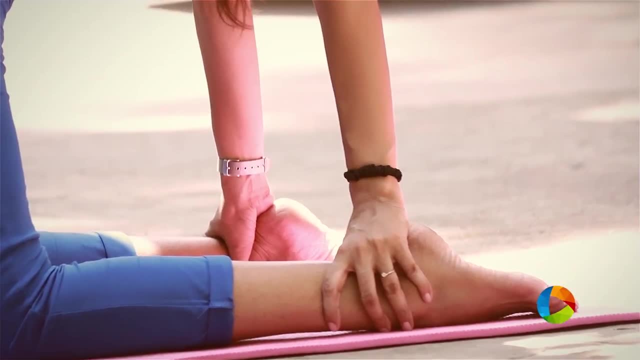 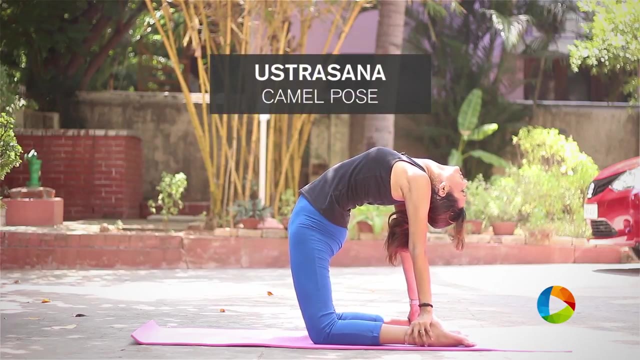 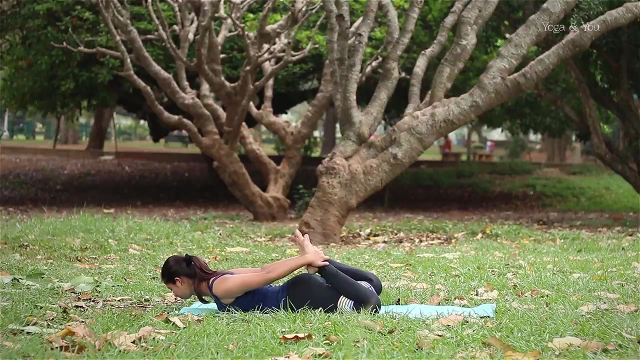 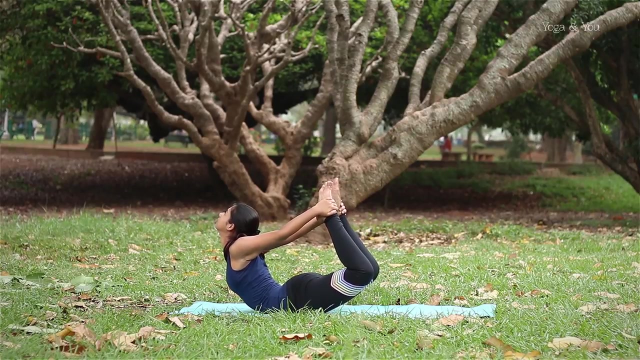 down onto the back of your hip and slowly inhale, first and exhale. slowly push your hips forward and slowly bringing your arms to your ankles and arch back. Lie down on your stomach, hold both your ankles and start to pull your ankles and lift your body up. If you look up, it will help you to go even higher. So the aim is to be on our 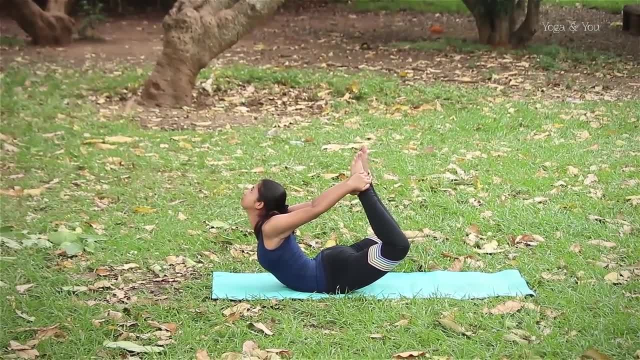 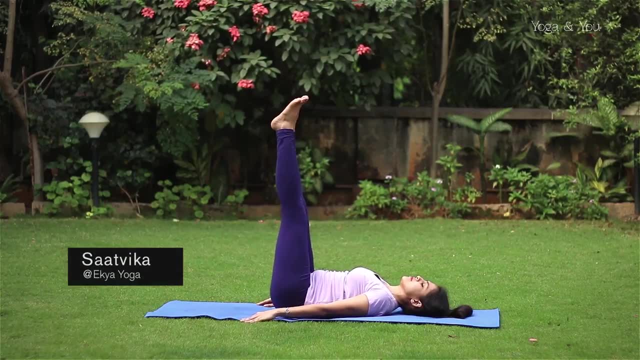 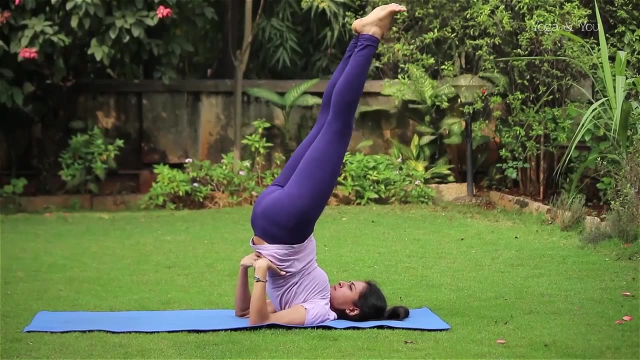 stomach, a whole chest, Everything, till the point of the ribs, should be up in the air From the supine position. raise your legs 90 degrees, Inhale, lift the feet and bring your, Lift the hips up and support your back. Come into sarvangasana.